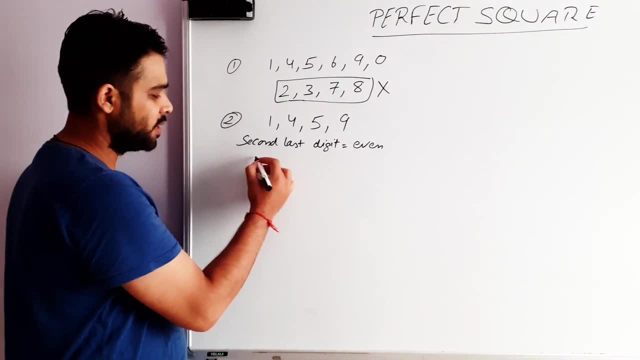 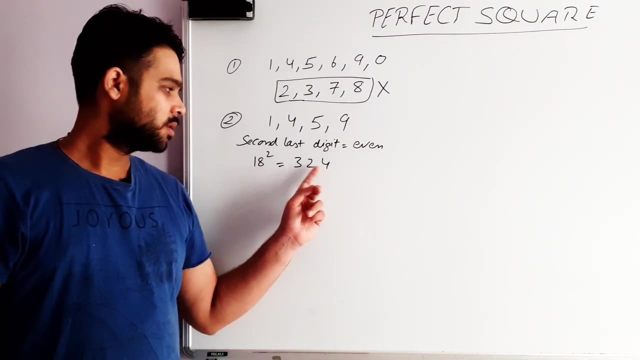 will give you an example. You take any random number and summary: it takes 18 squares. 18 square is 324.. You can see, here the last digit is 4, second last digit is then an even number. You take any random number. Now you suppose. 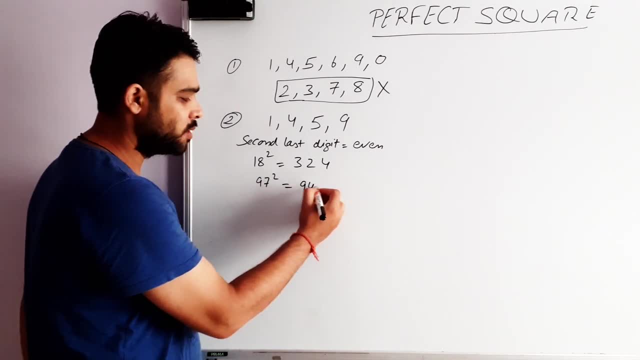 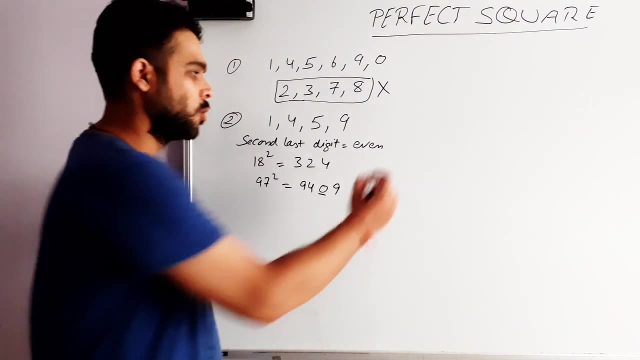 this is 97 square. 97 square is here 9,, 4,, 0,, 9.. This is basically the second last digit will either be an even number or zero- I will also write it- or 0.. Okay. 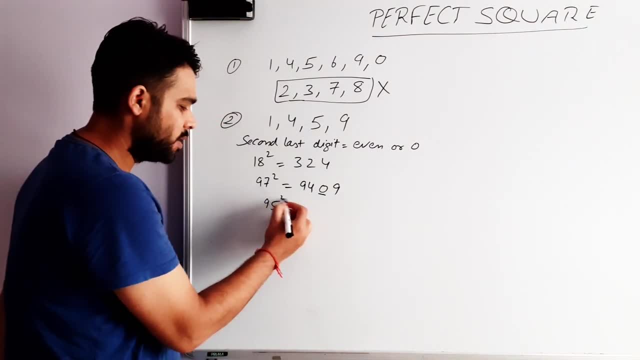 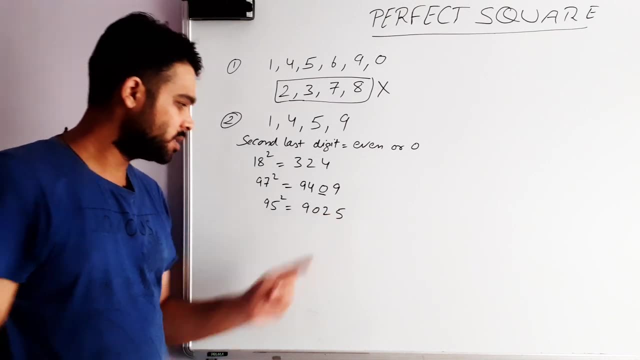 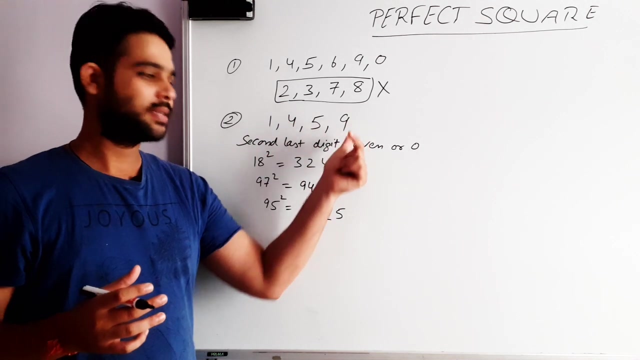 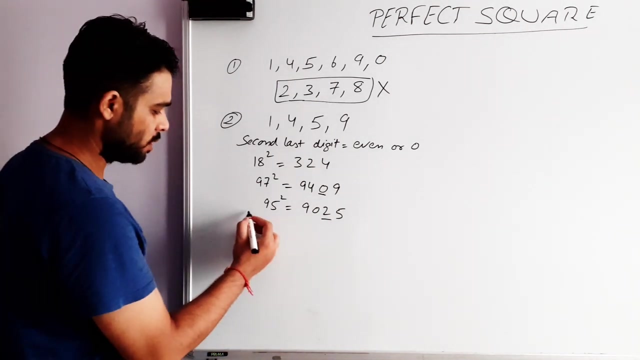 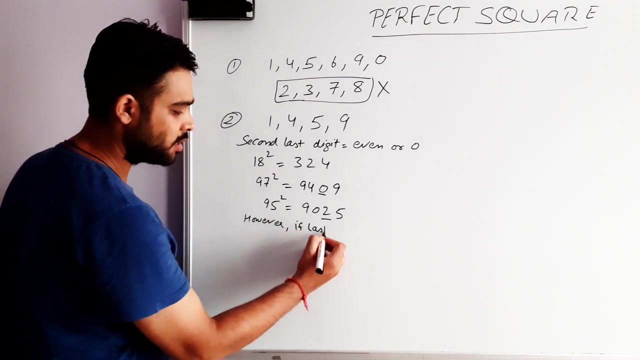 Now, if suppose you have 95 square, that is 9025. so the last digit was 5, your second last digit was an even number. you can see: whenever the last digit is either 1, 4, 5 or 9, the second last digit will be an even number. However, if the last digit is 6. however, if last digit 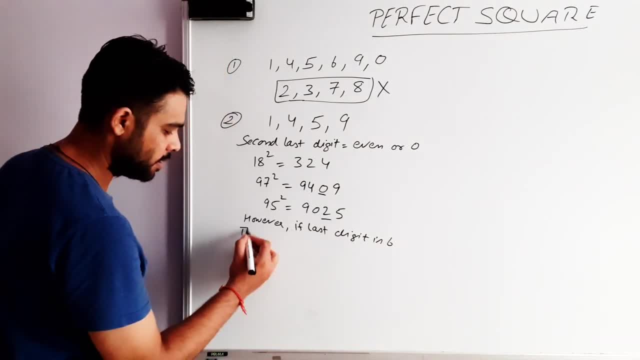 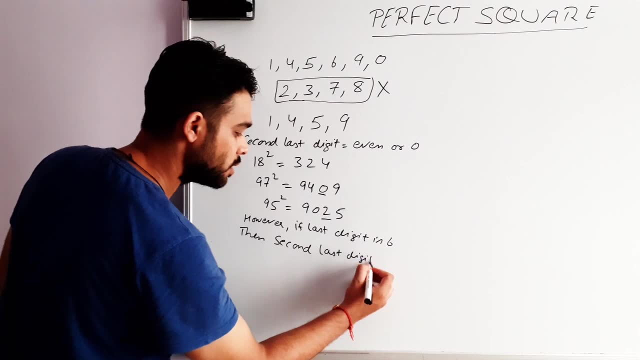 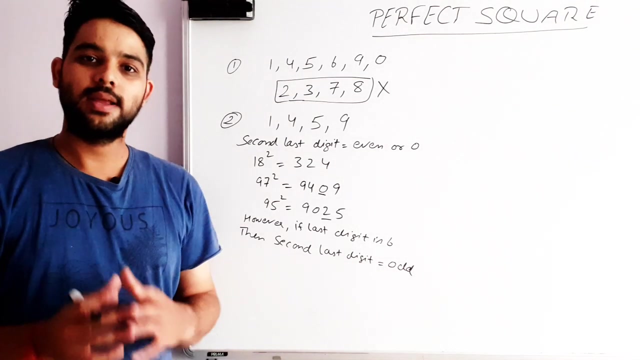 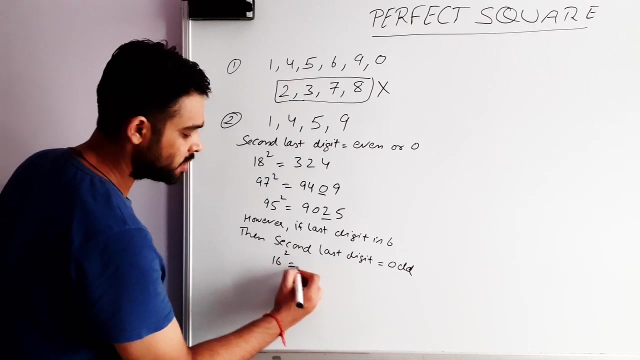 is 6, then second last digit will always be odd After 23 draws than second last digit will always be odd. we will take an example now. if suppose you are finding the square of 16, then 16 square is 256 last digit. 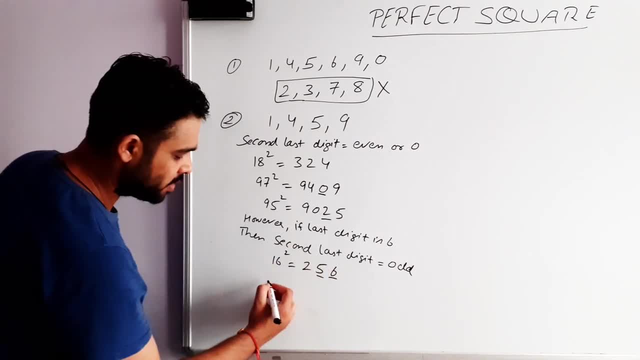 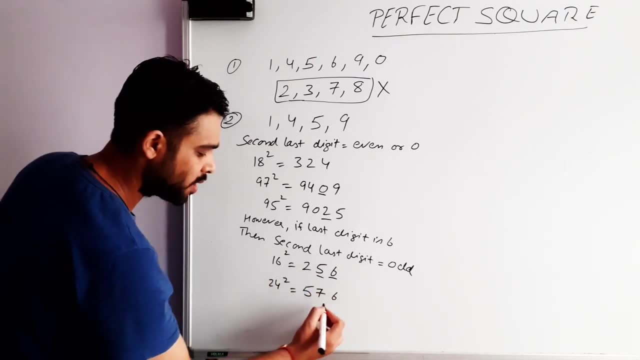 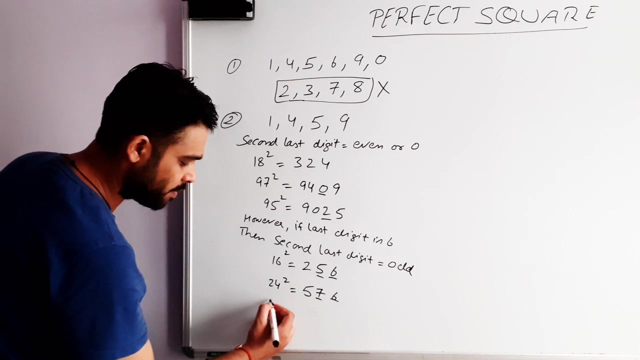 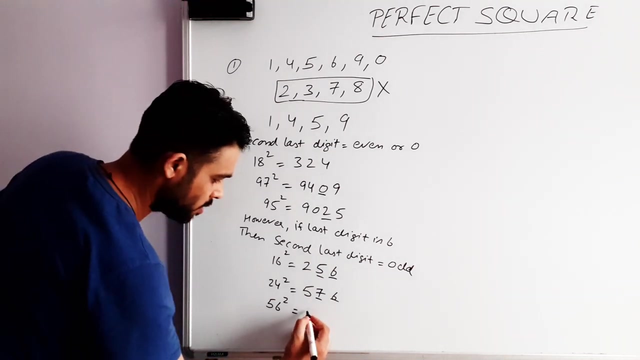 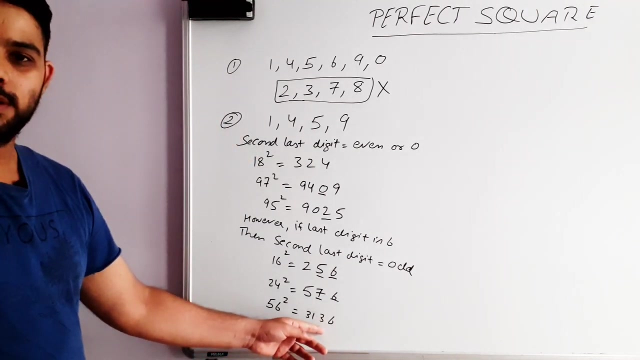 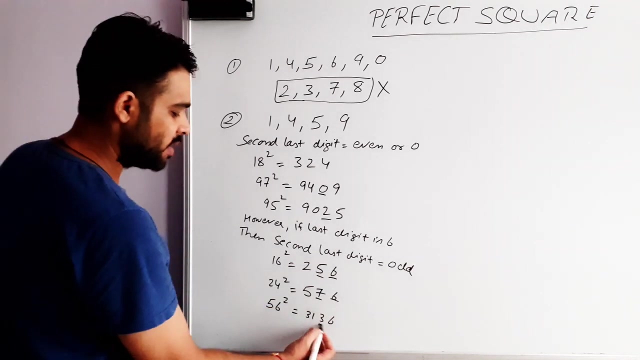 was 6, second last digit was an odd number. if suppose you are finding the square of 24, 24 square is 576. last digit was 6, second last it was an odd number. further, you are finding in and suppose then the answer is the second last digit is your odd number. So this is a very 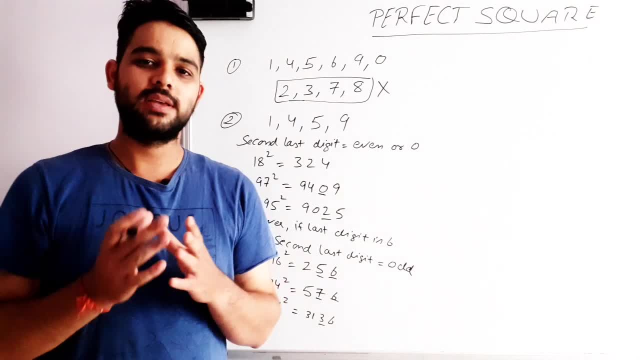 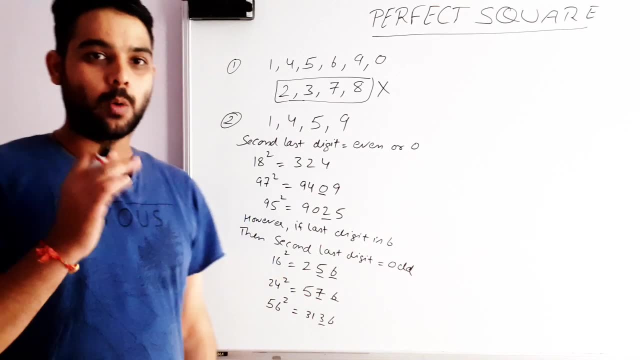 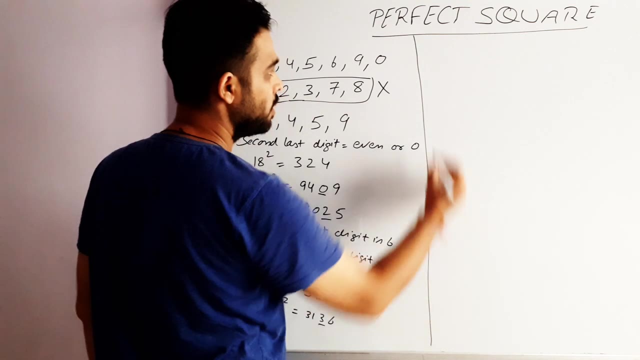 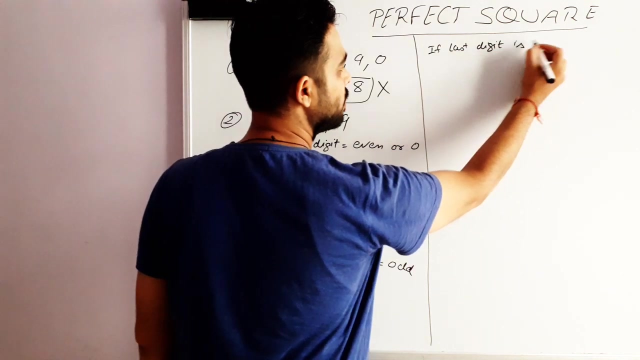 easy thing to remember. whenever you have the last digit as 1,, 4,, 5,, 9,, the second last digit will be an even number. but if the last digit is 6,, then the second last digit will be a odd number. Now one more thing: if the last digit is 5,, if last digit is 5, second, 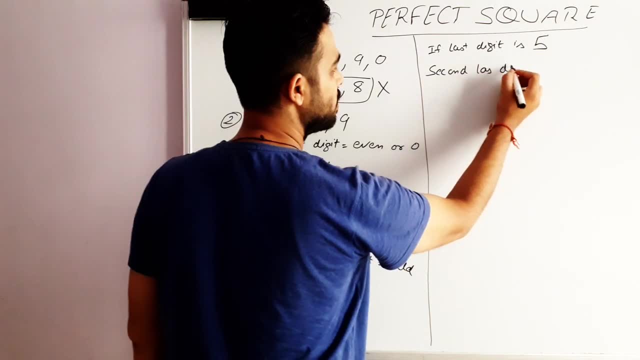 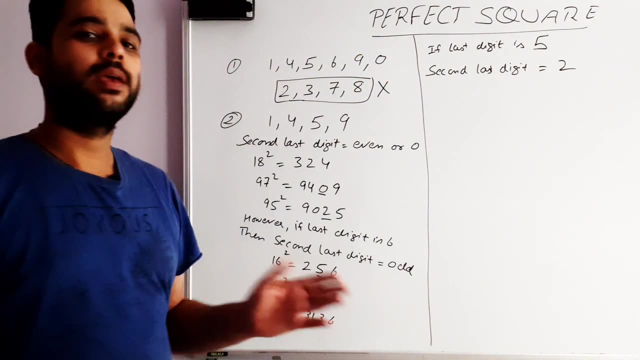 last digit will always be is even number. So if the last digit is 5,, then the second last digit will be equal to 2.. This means if you have 5 in the last, then the second last digit will always be 2.. For example: 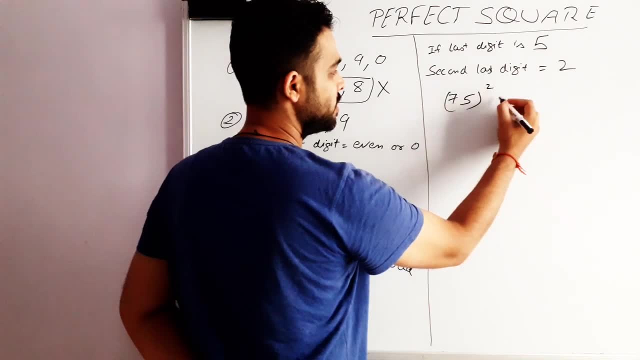 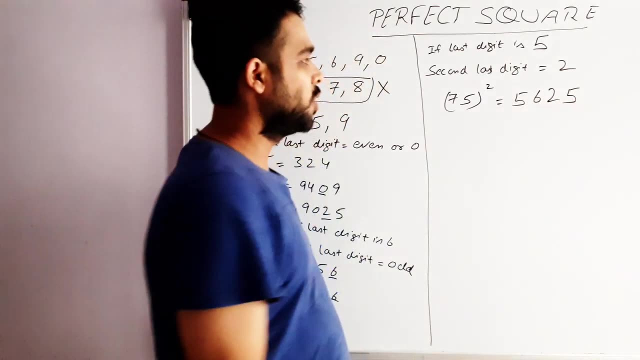 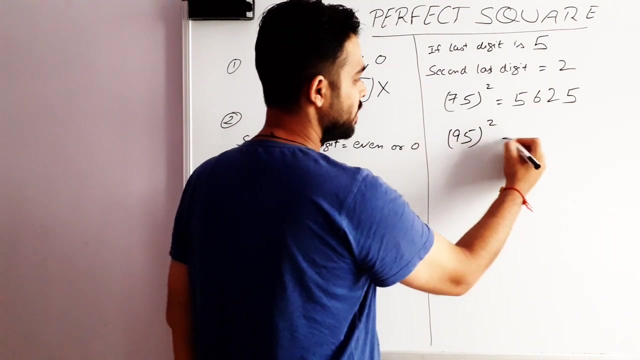 I will take the square of 75,. this is equal to 75. square is what? 5,, 6,, 2, 5.. So you have 5 and the second last digit is 2.. You take the square of 95, that is equal to 9025.. 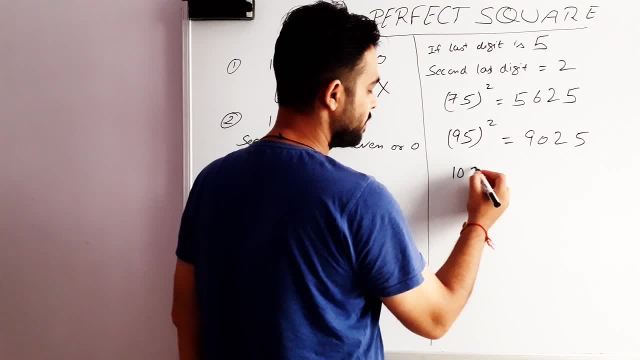 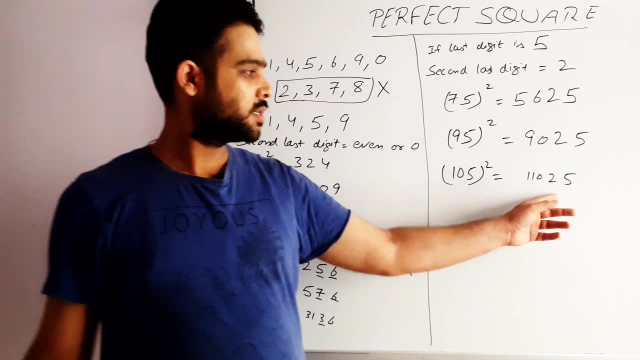 You take the square of 105, you will get 11025.. So the last digit is 2 in each and every case. You take any example. you take the example of 125, it is 15625.. The last digit will always. 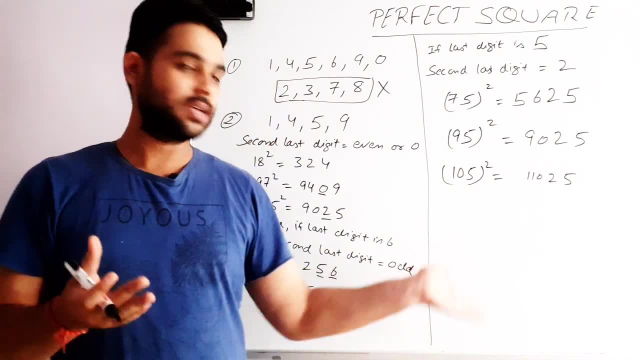 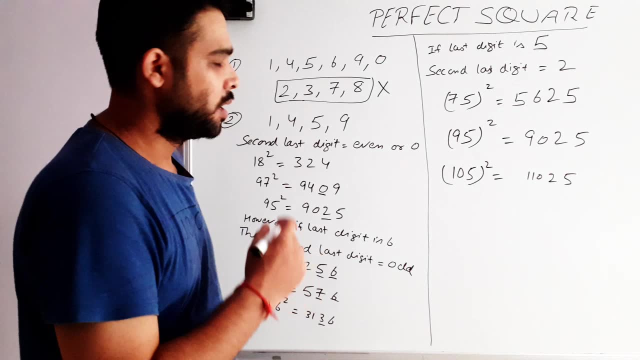 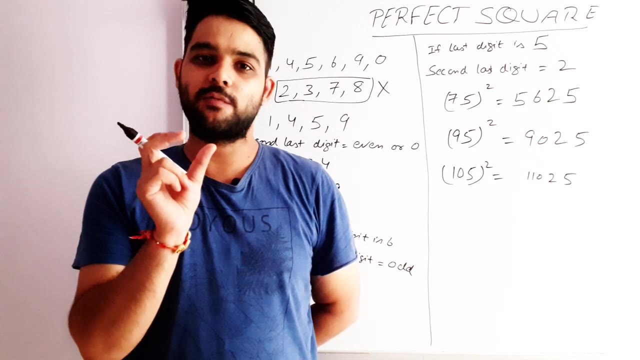 be 5.. Then the last digit is always 5, the second last digit will be 2.. Now coming to the most important part of this square: The digital sum of that perfect square will always be an odd number, or. 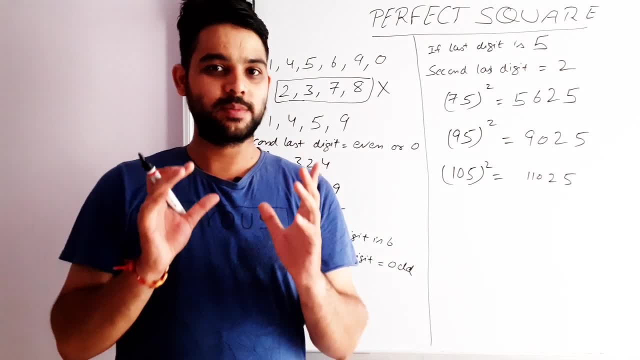 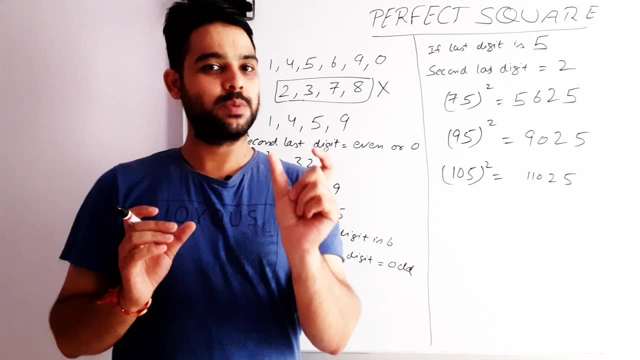 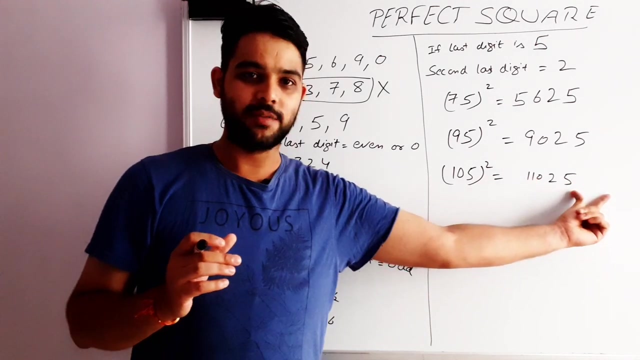 4.. Just try to understand what I'm saying. If there is a perfect square, the perfect square digital sum will always be an odd number, or 4.. What is the digital sum? Digital sum is basically the sum of all the digits that you are having For 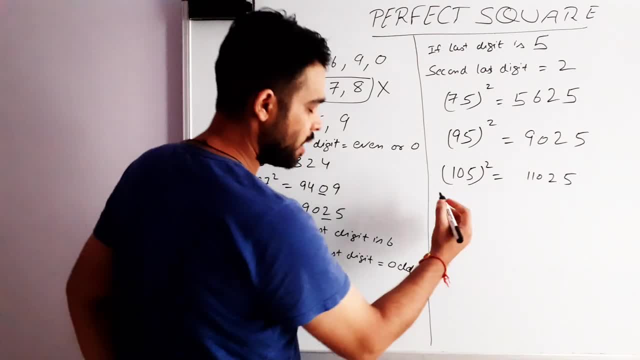 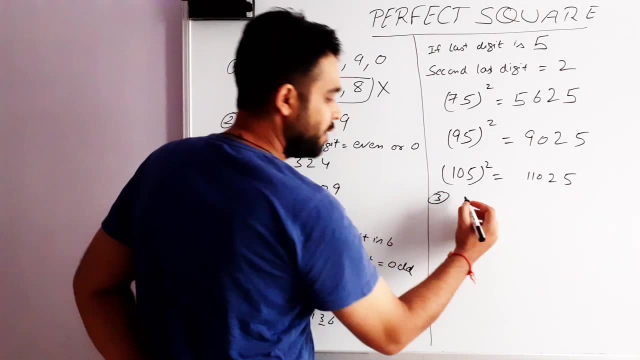 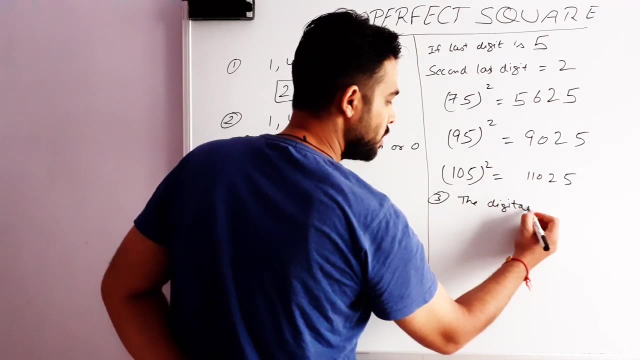 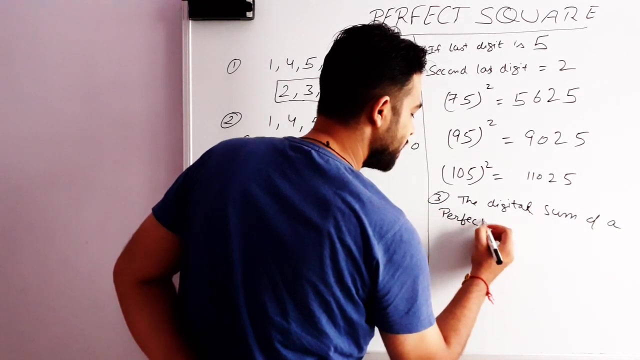 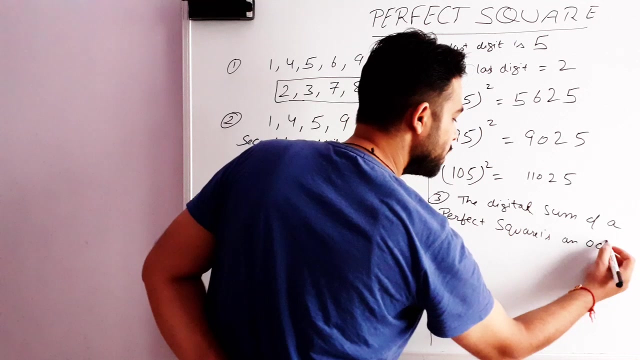 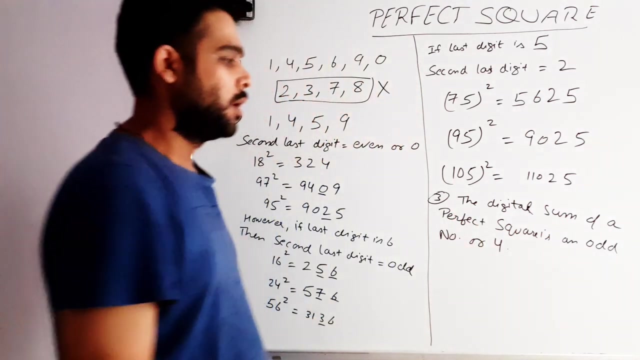 example. you take this example: 105 square. I'll write it down. write the quotation first. What is, what was that, If the digital sum, digital sum of a perfect square- is an odd number or 4.. Let's see it with an example. These all are perfect squares. You find the 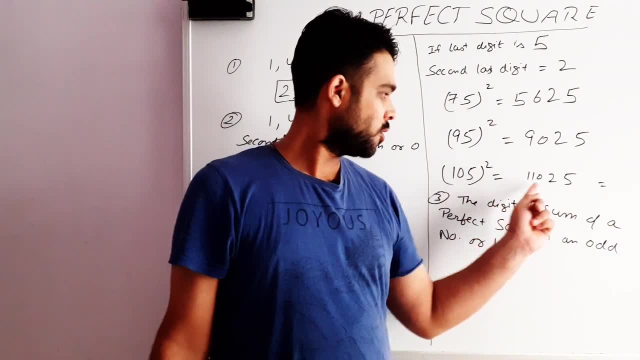 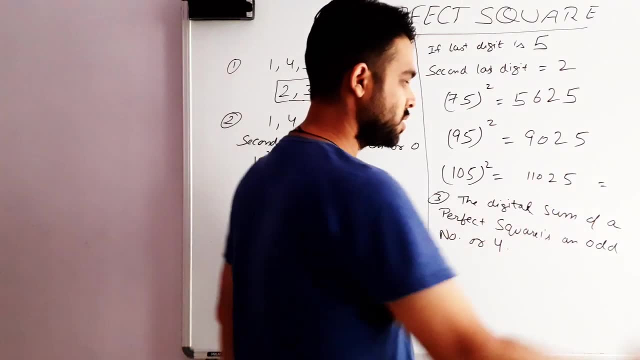 digital sum. For the digital sum, what I'll do is I'll add all these numbers. This is 1 plus 1, 2.. 2 plus 0, 2.. 2 plus 2, 4.. 4 plus 5, 9.. So the digital sum of this is 9, an. 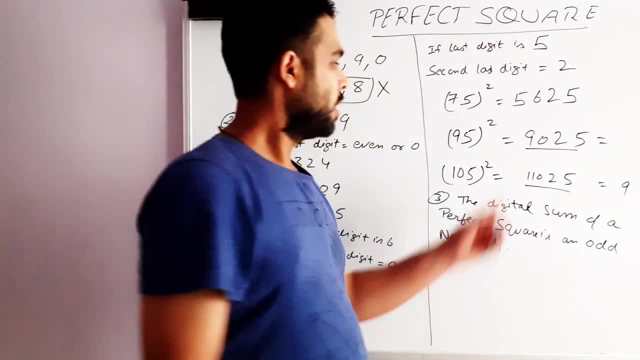 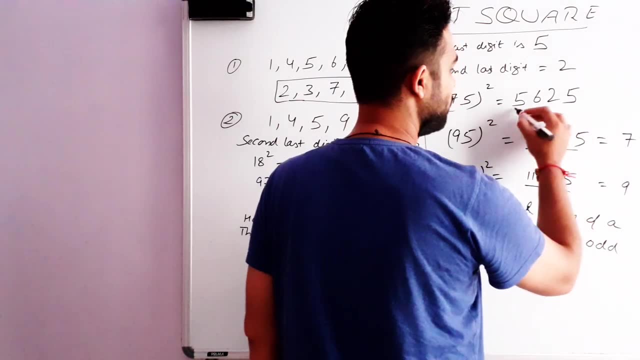 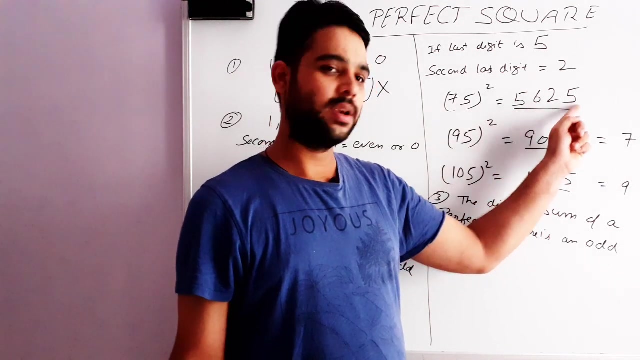 odd number: 9 to 11,, 11 and 5, 16.. 16 is 6 plus 1,, that is again 7.. You take the digital sum of this number, 5, 6,, 11,, 11 to 13.. 13,, 5, 18.. 18 is 8 plus 1,, that is equal to 9.. Again, an odd. 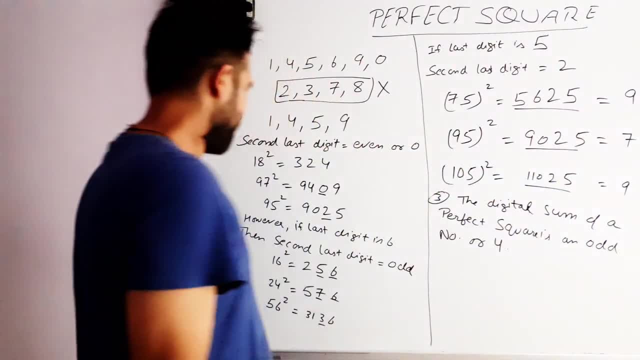 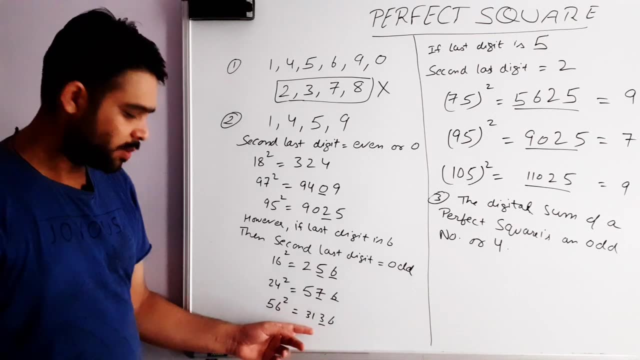 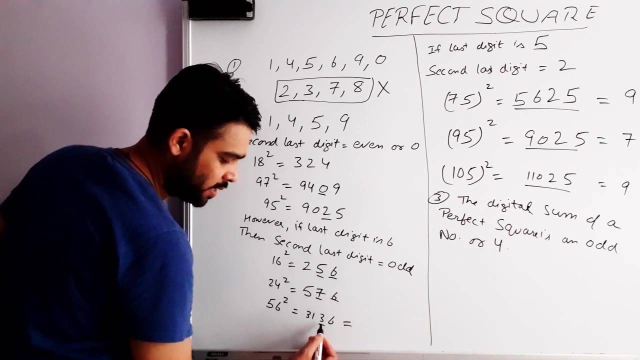 number. See this Digital sum of this number: 56 square. 56 square is 3136, 314, 437, 7 and 6 is 13,. 13 is 3 plus 1. that is equal to 4.. 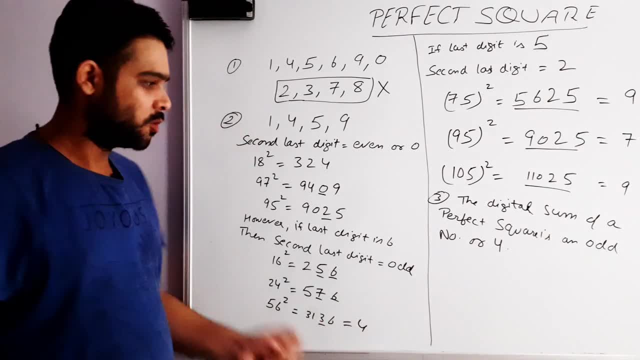 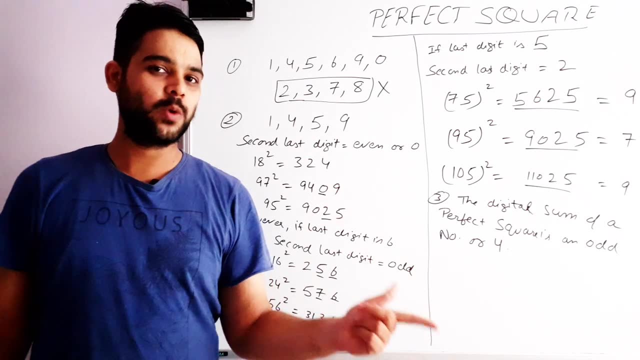 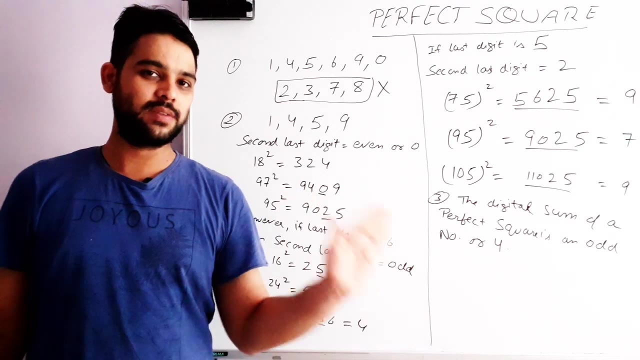 So the digital sum of 56 square is 4.. So you can see that the digital sum of a perfect square will always be an odd number and in the odd numbers it will never be 5.. This means it will take the values 1379 or 4.. 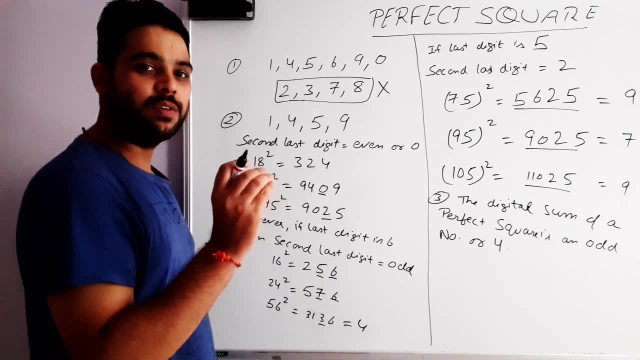 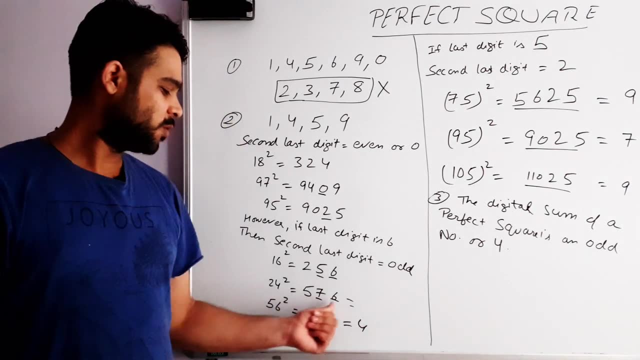 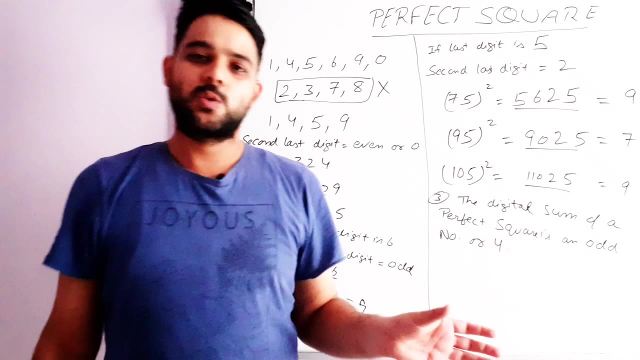 This is a very important technique and very easy way to find whether a number is a perfect square or not. You see the example this: 5712, 126, 18, 18 is 8 plus 1, 9.. You take any example, you take any perfect square, take its digital sum. it will always be an odd number or 4.. 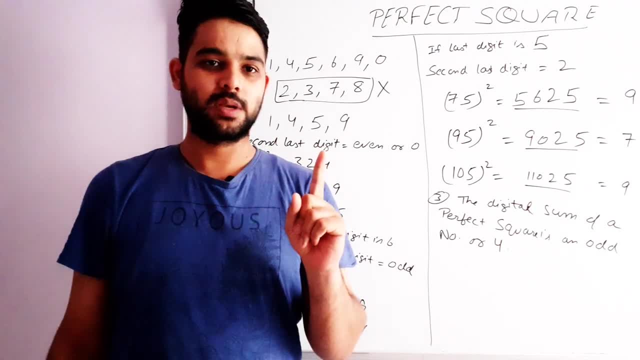 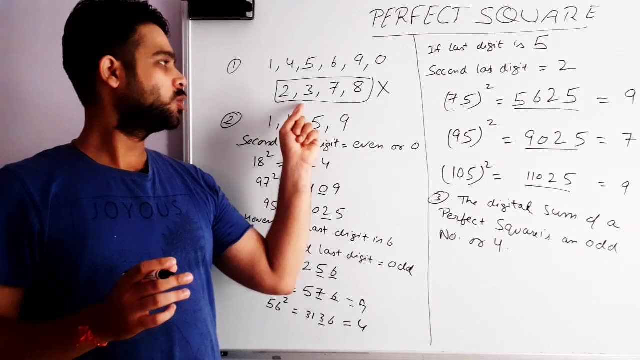 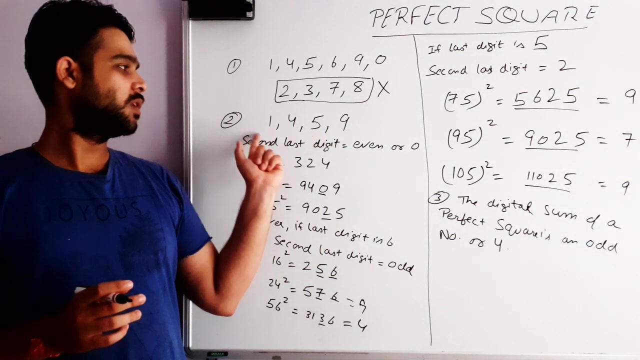 And also in an odd number, it will never be 5.. So to recapitulate what we have seen: A perfect square never ends in 2378.. The last digit of a perfect square will never be 2378.. Second thing, if the last digit of a perfect square is 1459, the second last digit will always be an even number or 0.. 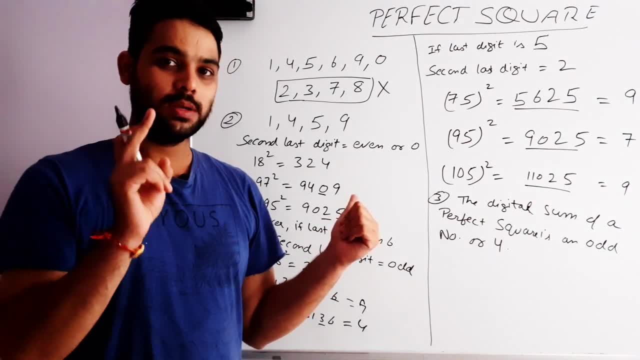 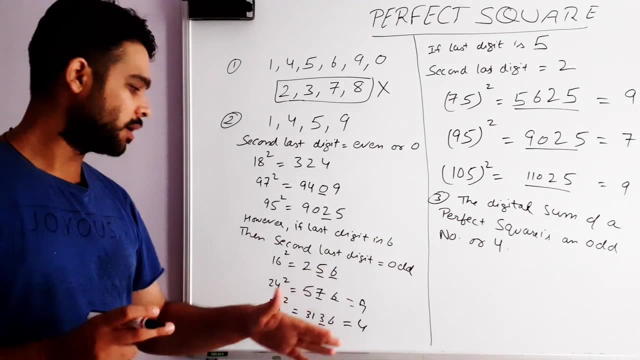 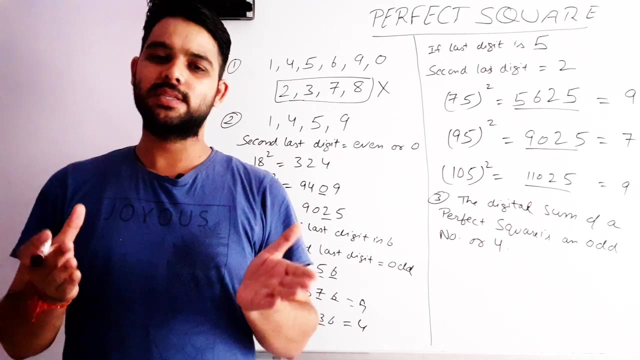 Second last digit will either be an even number or 0.. If the last digit of a perfect square is 6, then the second last digit will be an odd number. So if you, If suppose you are given a number 256 and 266 and they are asking you which of them is a perfect square,